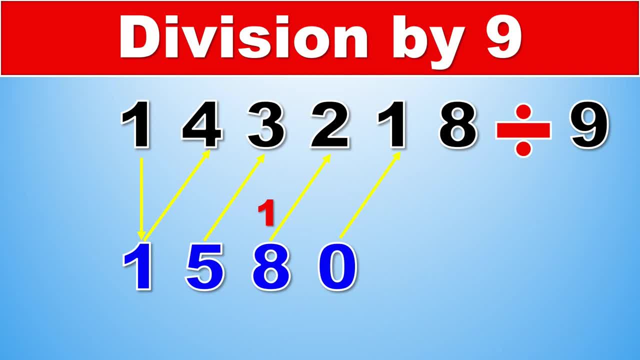 And so we carry on like this and go to 10 plus 1,, which is 11. And then again carry over the 1 and keep the other 1.. And finally we have 11 plus 8,, which is 19.. Now what we do is, instead of carrying over a digit, 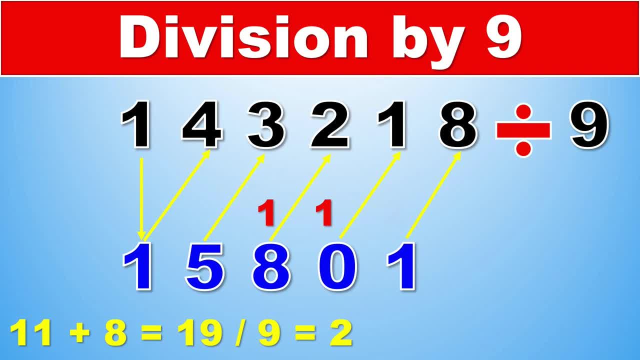 now what we do is we find out what 19 divided by 9 is, which is 2 remainder 1.. That means that we add 2 to the final digit and make the remainder 1.. Now let's finish up the rest of the quotient, Starting off with 1 plus 2, which is 3.. 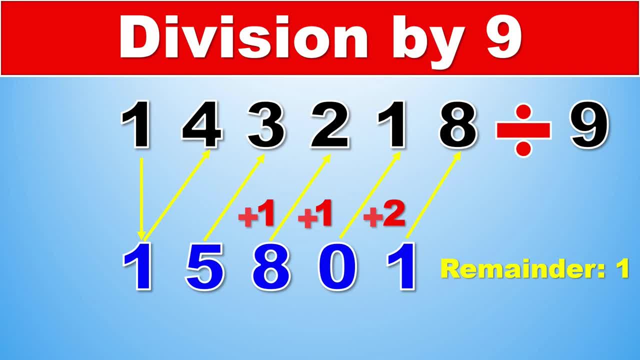 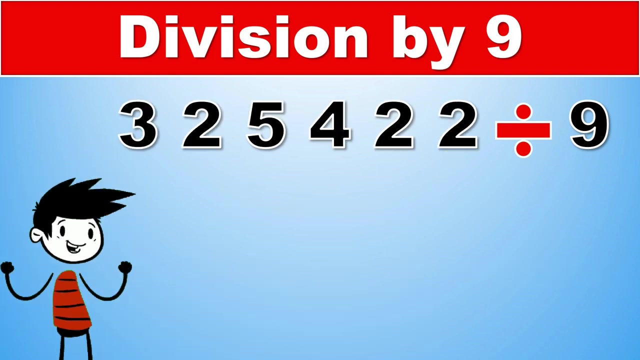 Next, 0 plus 1, which is 1.. 8 plus 1, which is 9.. 5 and 1.. And so we have it: 143,218 divided by 9 is 15,913.. Let's take another example: 325,422 divided by 9.. 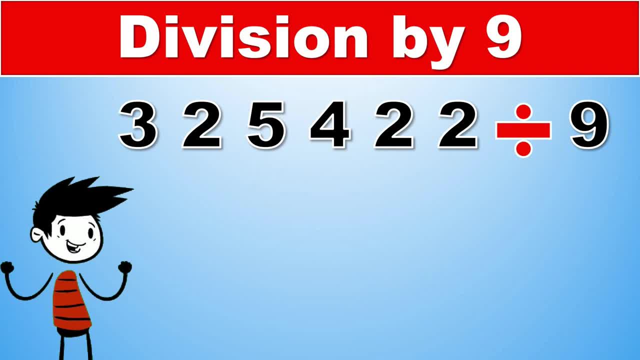 So let's begin Starting with the first digit of the number 3 plus 2.. We're next to a number 2 plus 1, and 5 andAAAAAAA, and which is 10. And so we have to carry over the 1 and keep the 0.. 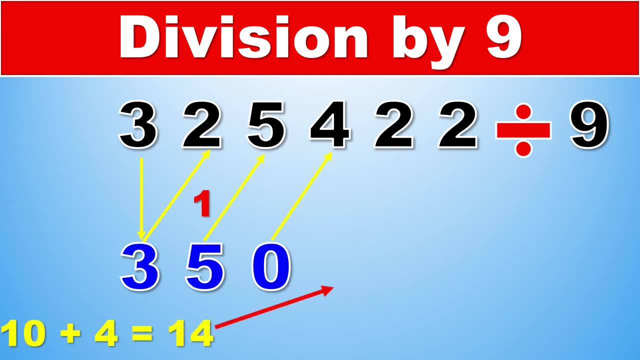 We follow the timeline going from 10 plus 4, which is 14. We're grants over to 5.. Moving on, 1 takes over the 10 plus 1, 14 plus 2,, 4, 1,. 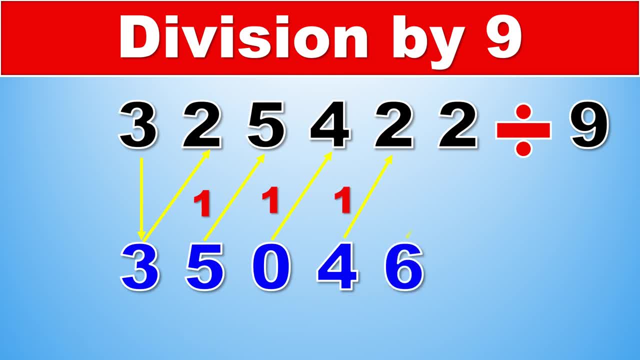 2, евой 줄 10, 6,, 5,, 2,, We have 16 plus 2, which is 18.. Now what we do with 18 is we divide it by 9, which is 2, remainder 0.. 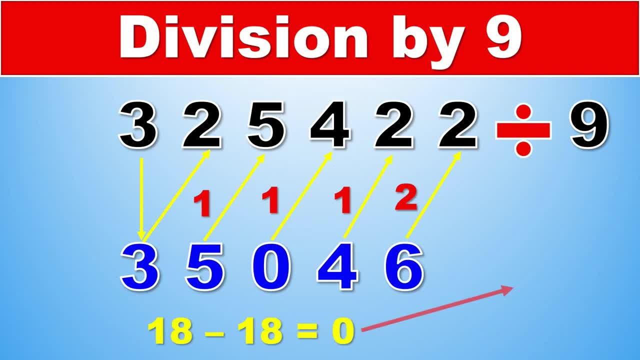 That means that we add 2 to our final digit and the remainder of the whole equation is 0.. So now let's finish up the rest of the quotient. So we have 6 plus 2, which is 8,, 4 plus 1, which is 5, then 0 plus 1, which is 1, and then 5. 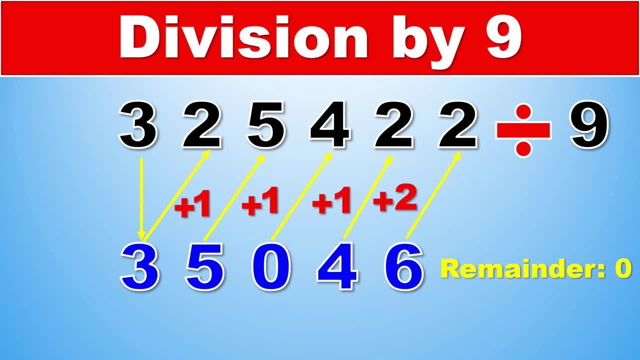 plus 1, which is 6, and finally, 3 is left as it is, Which means that 325,422 divided by 9 is 36,158.. And so let's go to our final number: 7,420,000.. 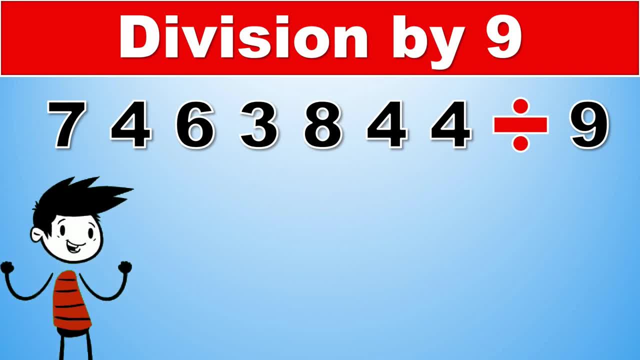 463,844 divided by 9.. Let's do this: Starting with 7 plus 4 is already 11.. So we have to carry over the 1 and keep the other one. Next we go for 11 plus 6, which is 17.. 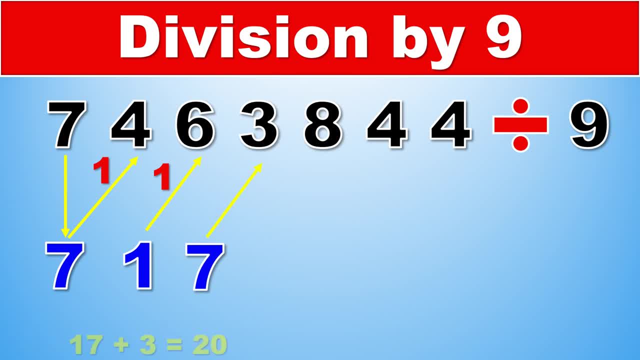 And then again we do the same. Carry over the 1, keep the 7. 17 plus 3 is 20.. So carry over the 2, keep the 0. Then we do 20 plus 8, which is 28.. 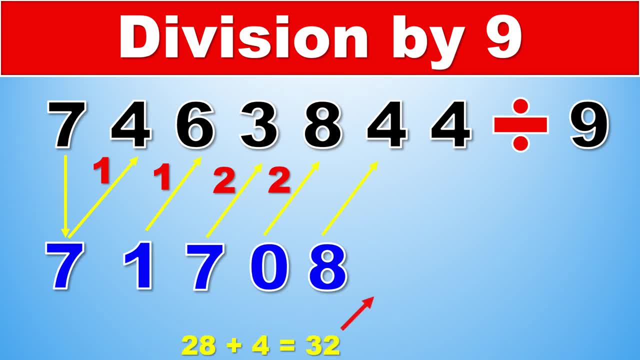 Carry the 2,, keep the 8.. Then 28 plus 4, which is 32.. So carry over the 3,, keep the 2., Then 32 plus 4, which is 36.. Now what we have to do is divide it by 9.. 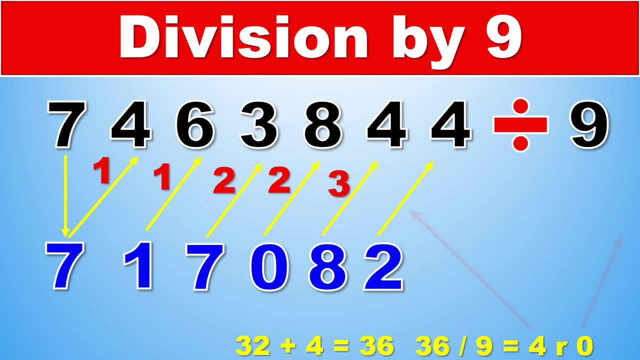 And 36 divided by 9 is very cleanly 4.. Remainder: 0.. Which means that 4 is the number that we add to our last digit and 0 is the remainder of the answer, Which means all we have to do now is just take a look at the remaining quotient. 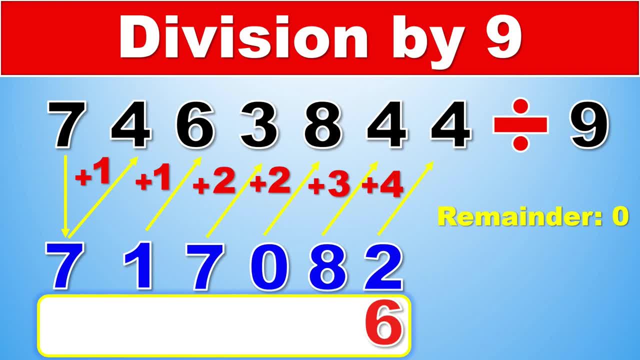 So we begin with 2 plus 4, which is 6,, 8 plus 3, which is 11.. So this time we have to carry over again. Carry over this 1 to the next one, which is 0 plus 2.. 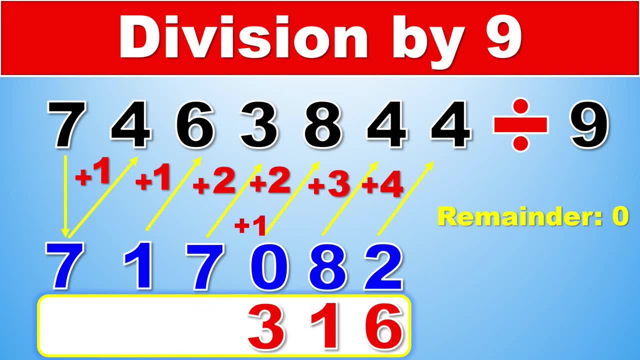 Add the 1 there and it becomes 3.. So that's the 3 there. Next we have 7 plus 2, which is 9.. Then 1 plus 1, which is 2.. And finally 7 plus 1, which is 8.. 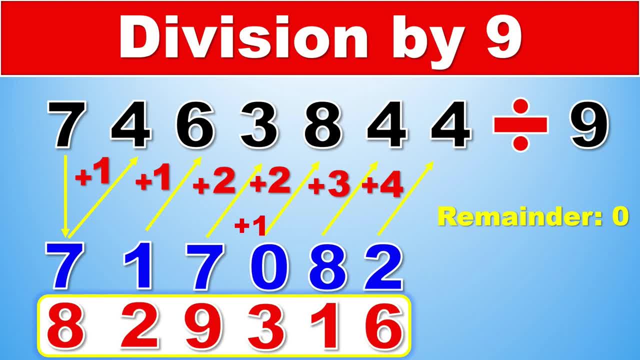 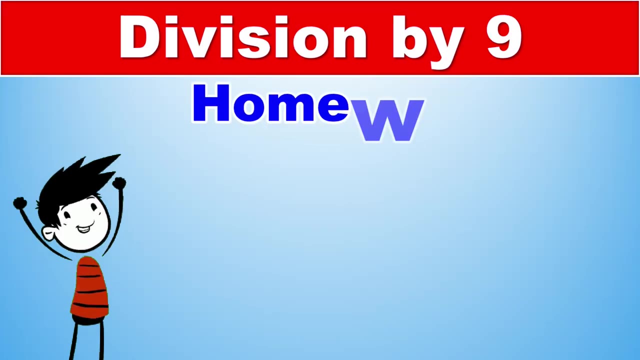 Which means that 7,463,844 divided by 9 is 829,316.. And that is the division by 9 trick. Now that you know this trick on how to divide any number by 9 easily and quickly, here is some homework.